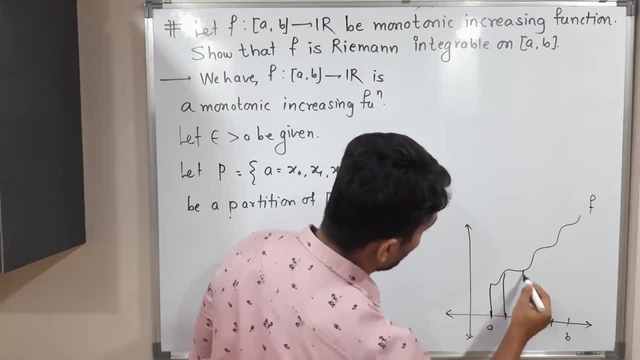 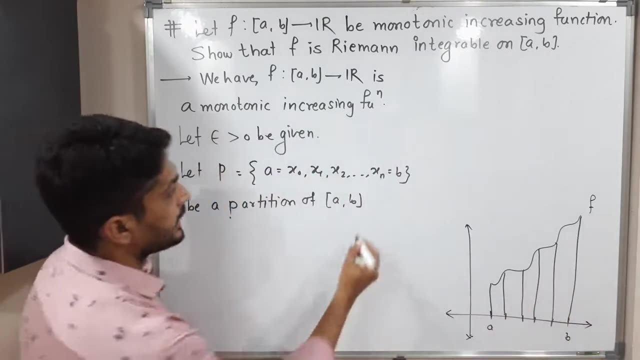 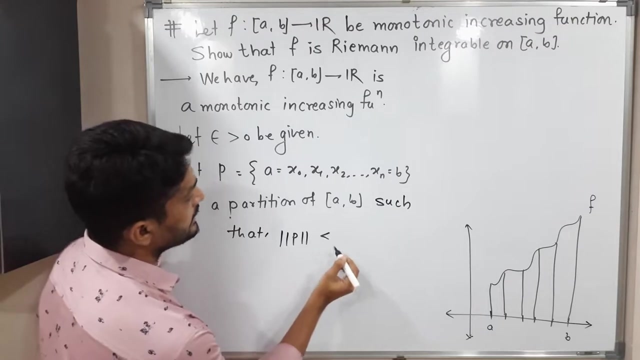 partition like this: So because of this partition, region will be divided into, yes, these parts. I am drawing a rough sketch here, Okay, Okay. So such that I am adding one condition, Such that- So that condition is norm of partition- is less than epsilon by f of b minus f of a. 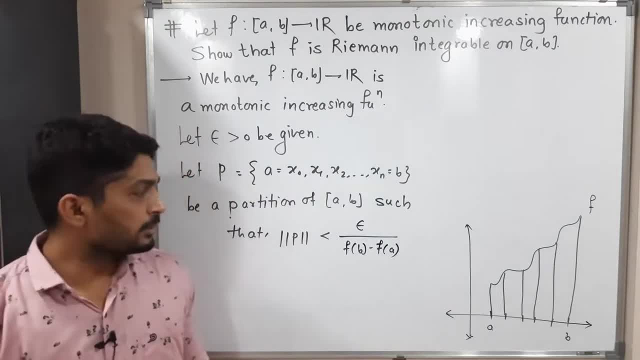 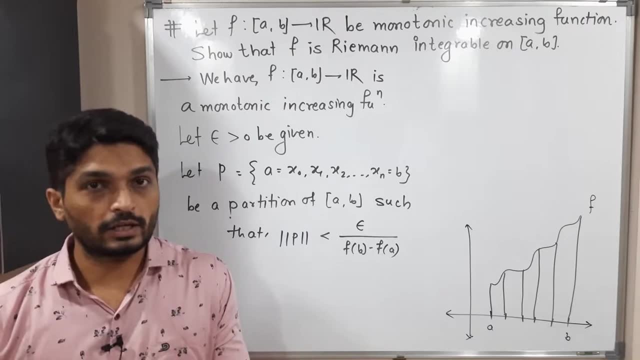 Epsilon by f of b minus f of a. So maybe you will get confused. What is meaning of norm p? Norm p, that means norm of any partition that is nothing but length of, okay, largest subinterval. That means see, because of this partition, the main interval is divided in subinterval. 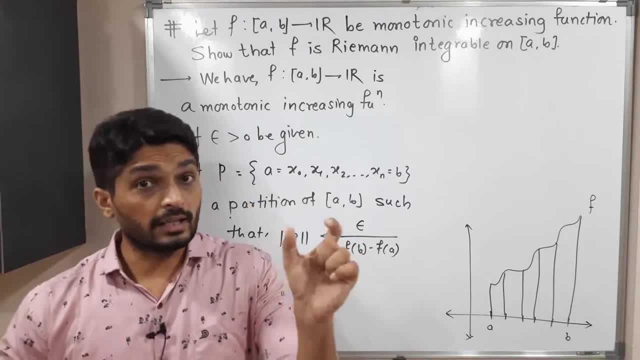 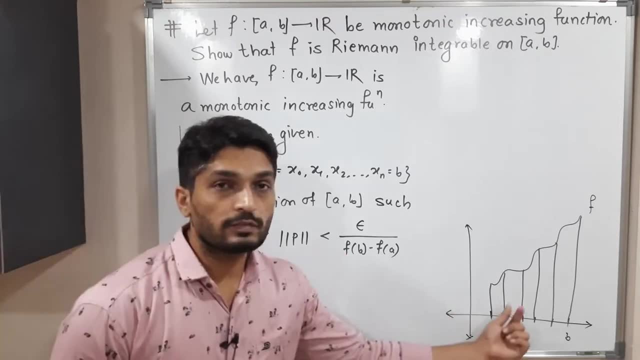 So we will find a largest interval And its length is nothing but norm of a partition, See norm of p is less than this one. That means length of each subinterval is less than epsilon by f of b minus f of a. So this: 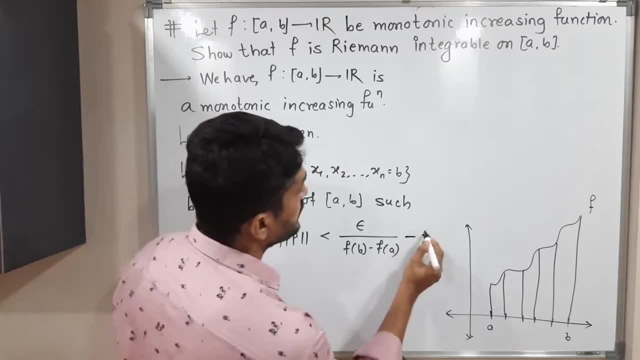 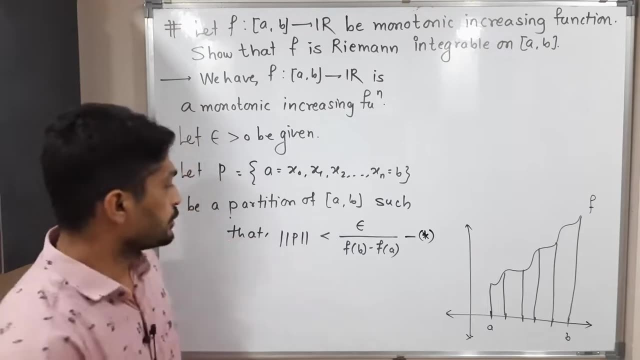 is a very important part of our proof, So let me call it as star. Let us go further. So after that, we will define capital mi, We will define small mi. So now now, capital mi. So I think you are familiar with definition of capital mi, So let us go further. So. 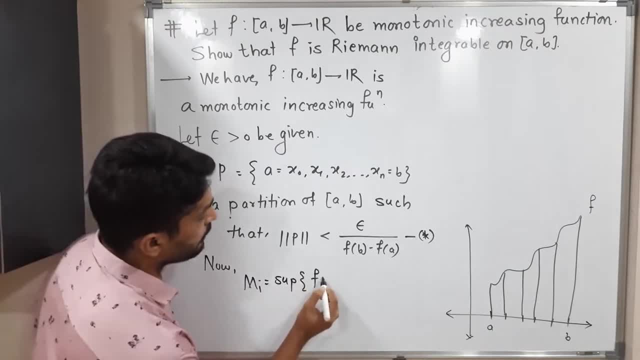 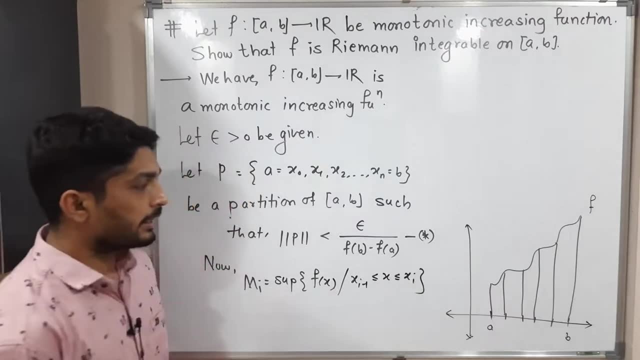 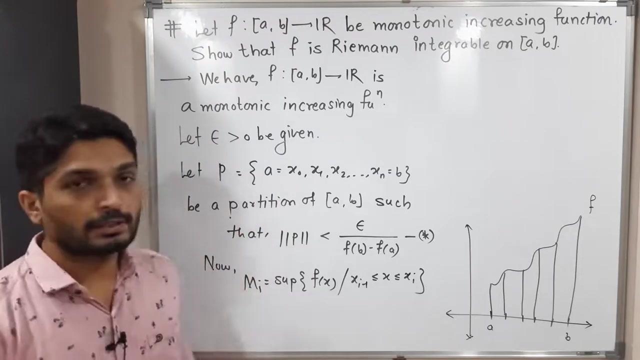 which is equal to supremum of supremum of f of x, such that xi minus 1, less than or equal to x, less than or equal to xi. That means in each interval, okay, or each subinterval function has some maximum value. that is nothing but capital mi. But see, the function is increasing. 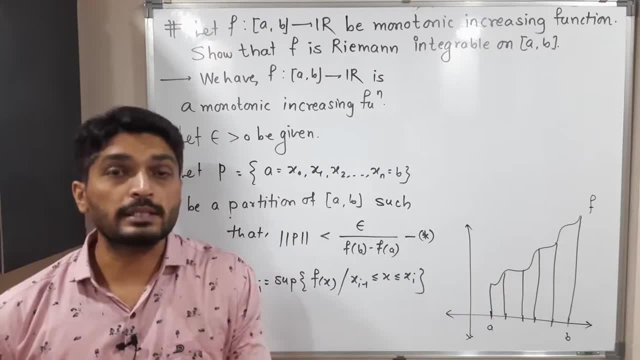 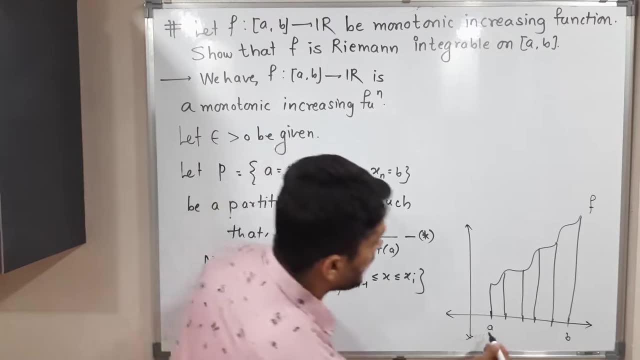 okay, function is increasing, So that is why function will have its maximum value at right end of an interval. Let us see, for example: if you consider the fourth interval, A, that means x0, this is x1, x2.. If you consider the first interval: x0, x1.. So function? 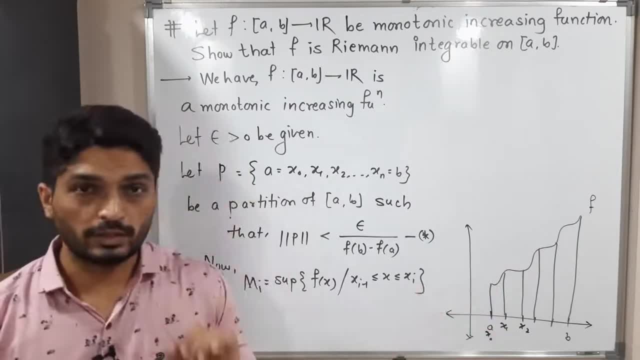 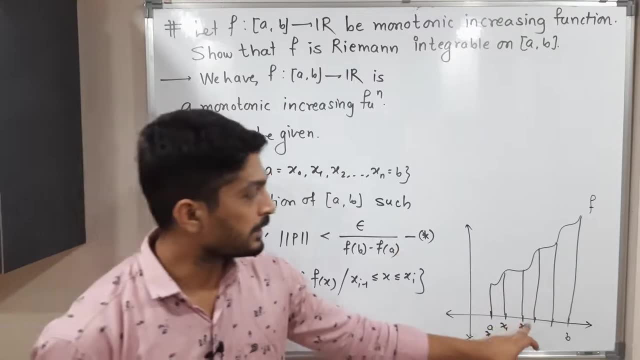 is increasing. So that is why it will have maximum value at x1.. If you consider the second interval, as function is increasing, it will have the maximum value at x2.. Similarly, for next interval, function will have the maximum value at x3, and so on. That means at right. 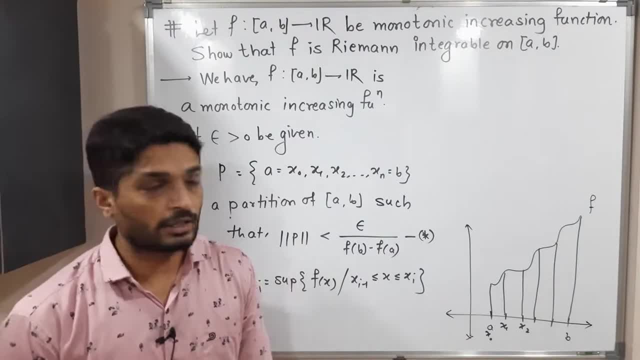 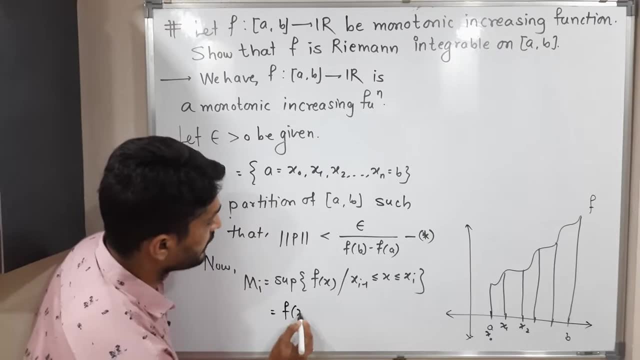 end of each interval, function will have its maximum value. So here also same thing will happen. So right end of interval is xi. So function will have maximum value at xi. So I am writing f of xi. Let us go further Now. 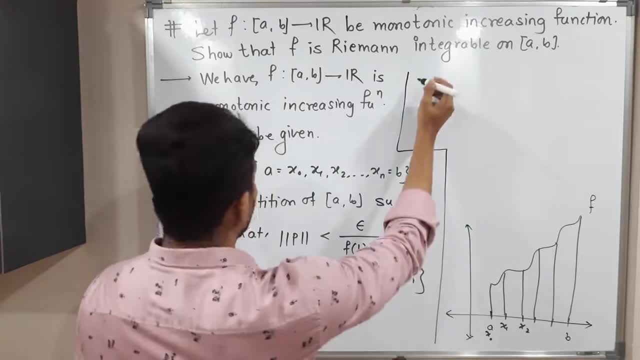 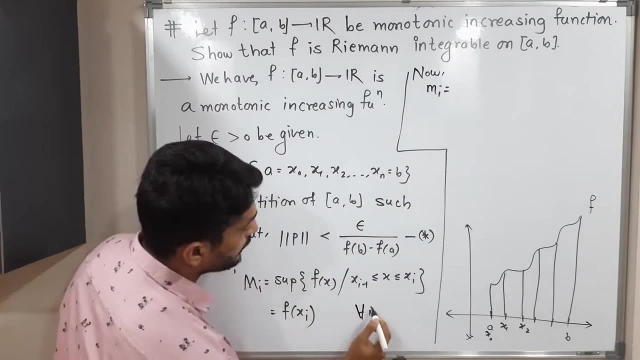 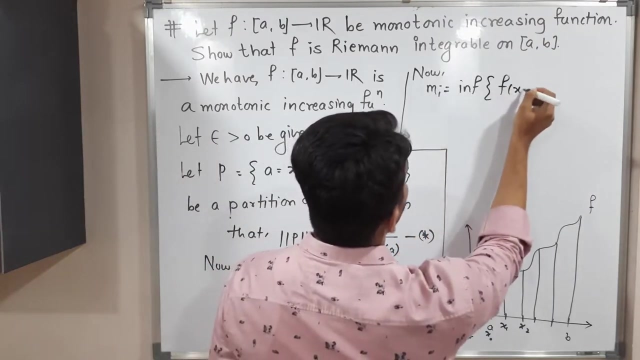 we will define small mi. Let me mention here Now small mi. Will you tell me the definition of small mi? So obviously I should write for all i running from 1 to n, that thing I should mention. Small mi is int of f of x, such that xi minus 1, less than or equal to x, less than or equal. 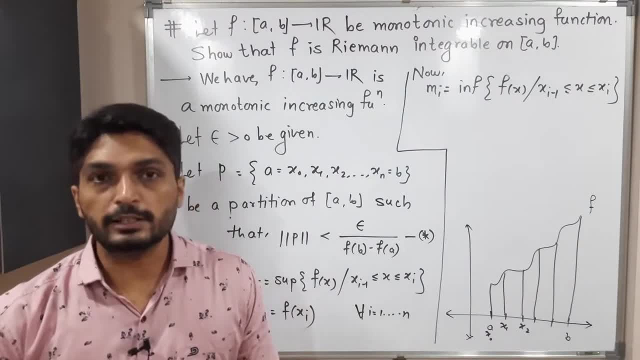 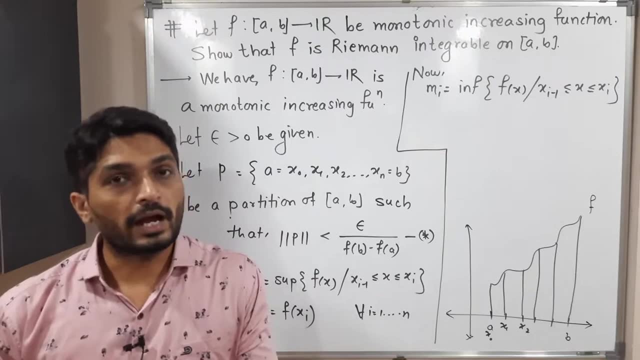 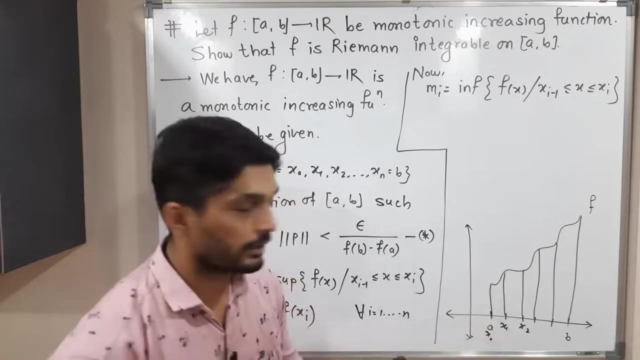 to n i, which is the minimal function at an interval, Since function is increasing. So if you take minimum value at x0 or x1, theion of x1 is at least an interval. Do you see that? Then it will be again small mi. Now if I write at x1, i will get the minimum value. 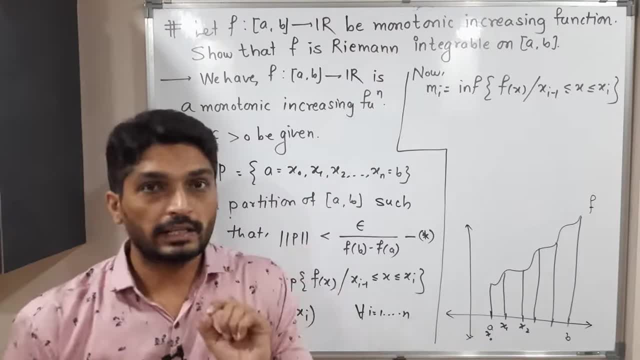 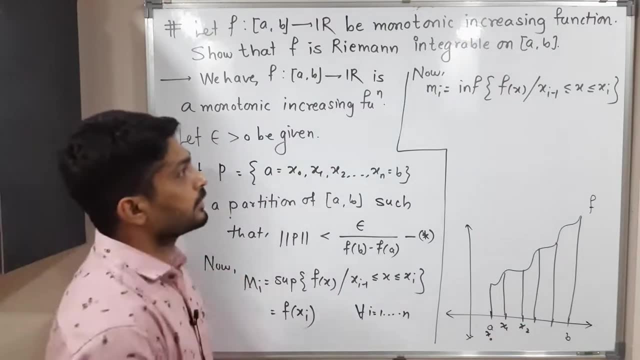 at x1.. So in this way you will see everyone trying to write in c1.. That means the minimum value you are given at x1 are the minimum value for that interval. Okay, So Section ñ of function is at미 ridiculous. Next time we will see about reaction time At which. 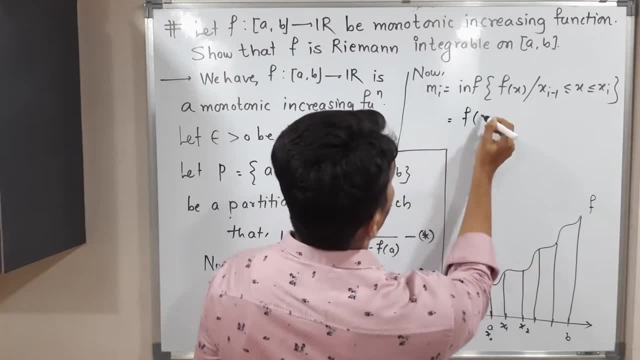 time you are getting the minimum value of function at x1.. So if you talk about, the first interval is xi. So it will have the maximum minimum value at xi. Okay, xi minus 1, f of xi minus 1.. So here, 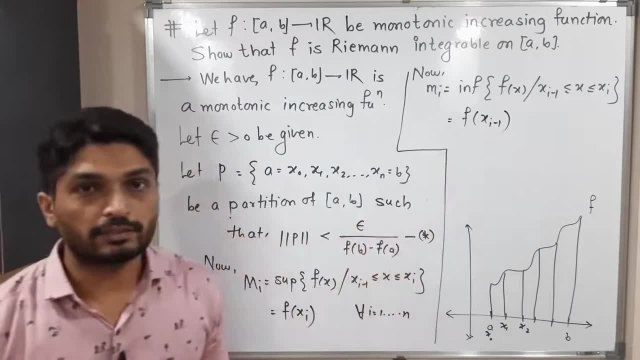 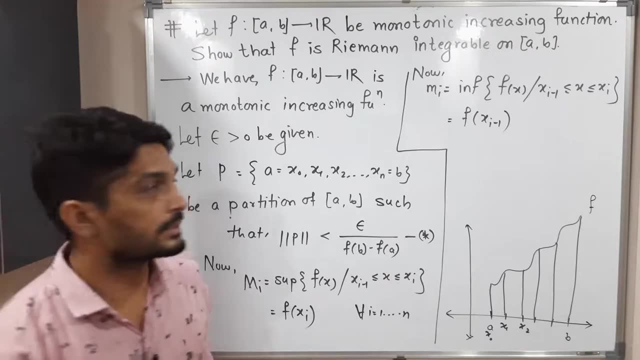 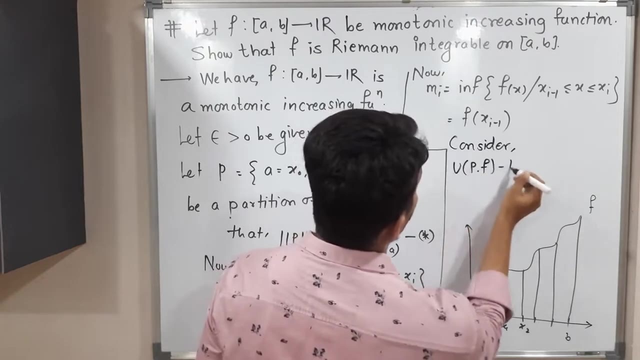 we have at the right end and here we have at the left end. Let us go further. After that, what will I do? I will consider upper integral, upper sum minus lower sum. Let us see. So consider I am considering upper sum, upf minus lpf. Okay, I should mention here for all i running from 1 to n. 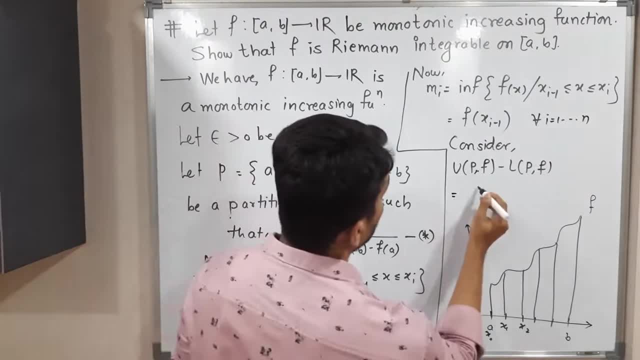 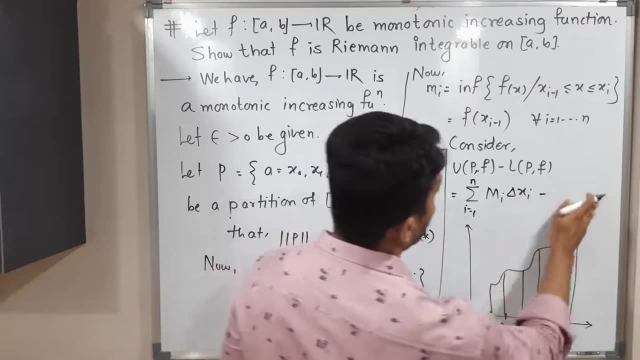 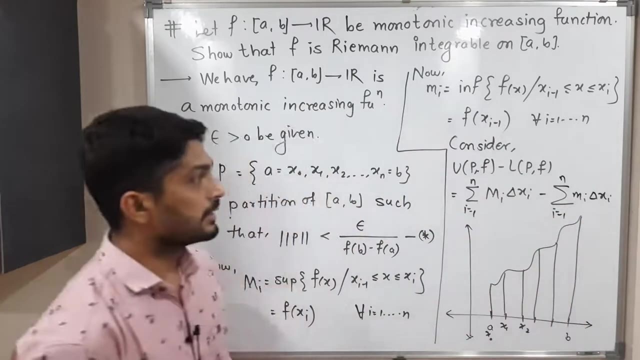 Let us put their values. What is the definition of upf? That is summation capital mi delta xi i running from 1 to n minus. let me mention here summation i running from 1 to n small mi delta xi. See, if you try to subtract, what will happen. 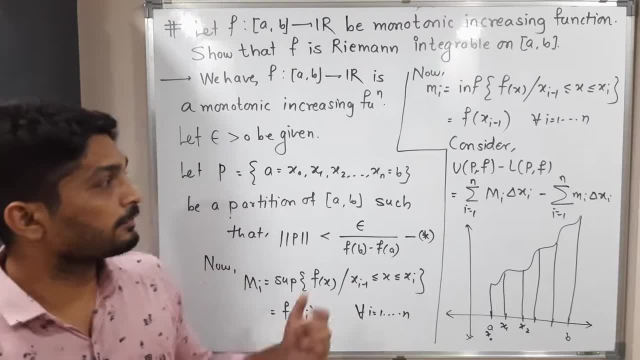 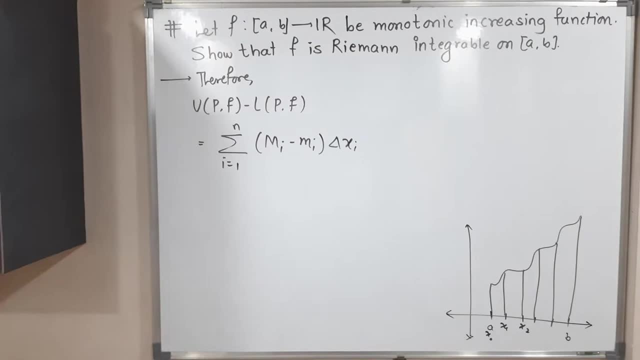 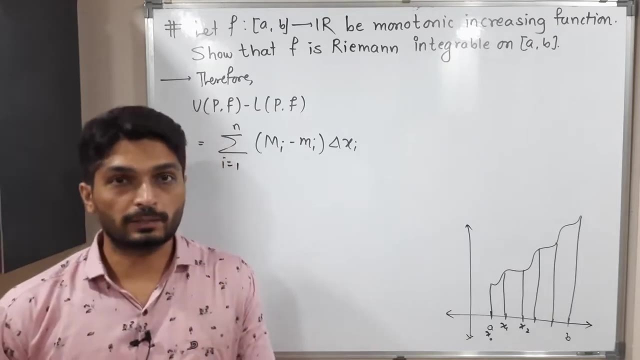 See, we can take summation common, we can take delta xi common and we can write capital mi minus small mi. Let me write that thing. So by taking summation and delta xi common, we will have this one. But will you tell me what is delta xi? Delta xi means length of each interval, See length of. 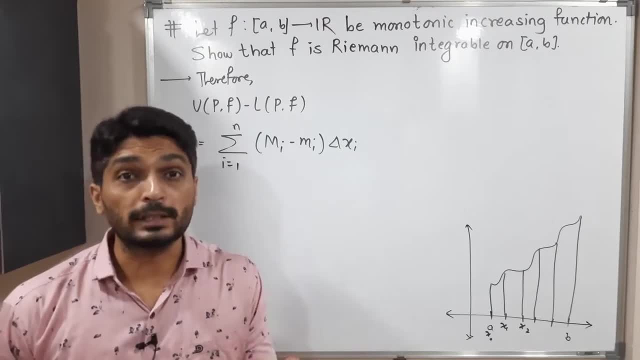 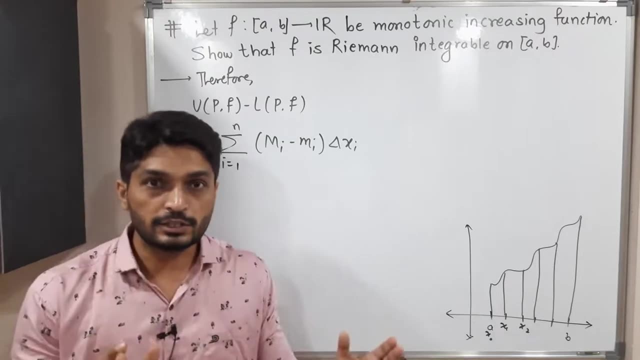 each interval is obviously less than or equal to norm p, since norm p means length of largest interval. So length of each interval is always less than or equal to length of largest interval. Okay, So we have this small, smaller intervals, So we are talking about it, So we can write less than. 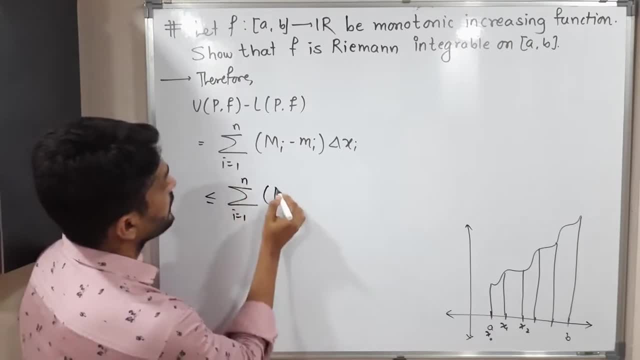 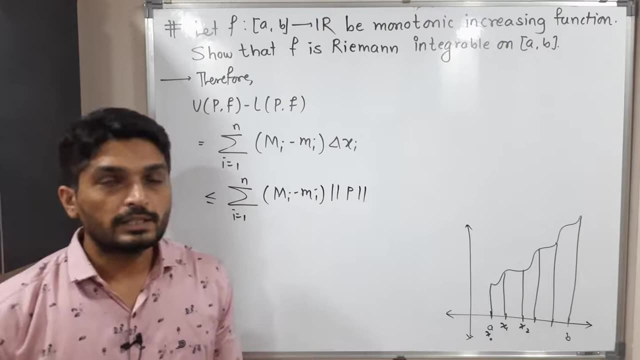 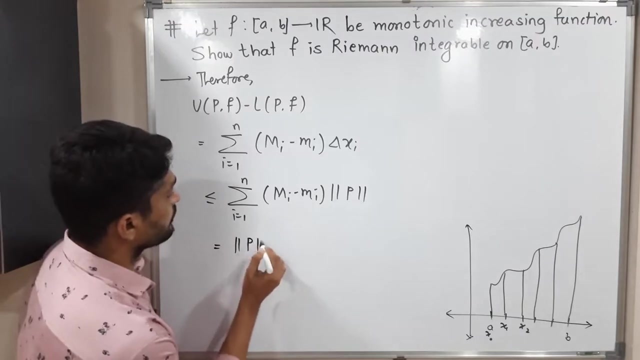 or equal to summation i running from 1 to n capital mi minus small mi. norm p, Since delta xi is always less than or equal to norm p, So that norm p is independent on i, So we can take it outside. So this is equal to norm p summation i running from 1 to n capital mi minus small mi. 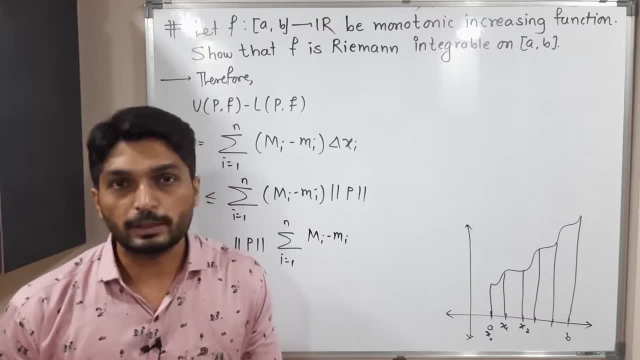 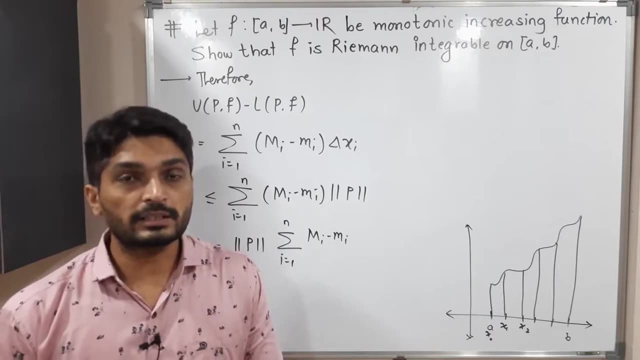 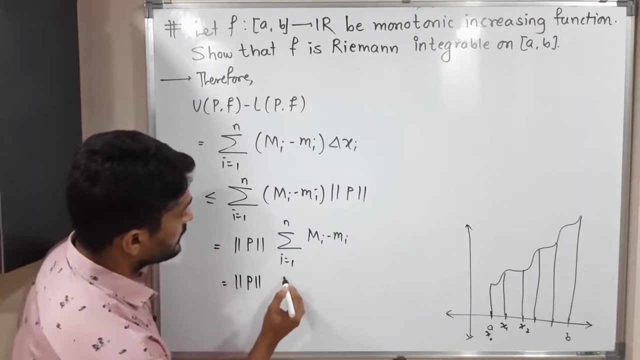 Do you remember? already we have found out the value of capital mi and small mi. Capital mi is nothing but f of. do you remember that is f of xi and small mi is nothing but f of xi minus 1.. So let us put their values here. So this is equal to norm p. Okay, Summation. i running from 1 to n. 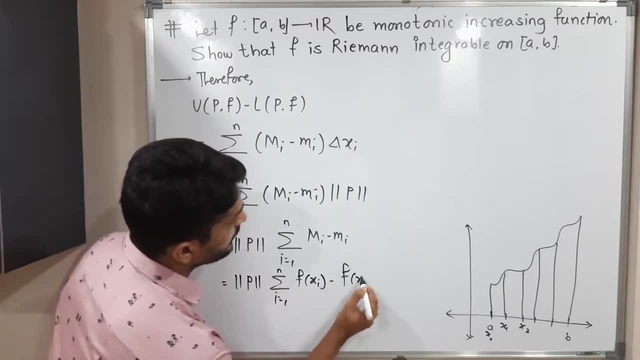 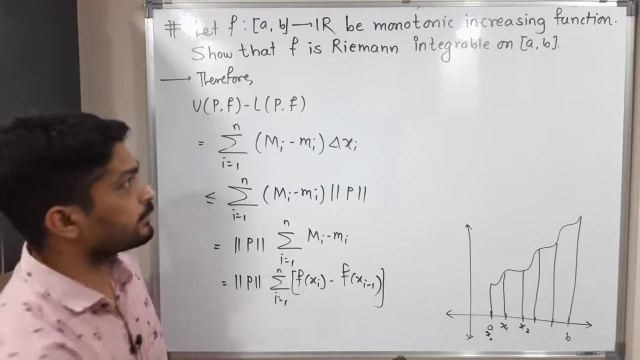 f of xi minus f of xi minus 1.. So will you guess what I'm going to do? Yes, I'm going to expand this summation. Let us see what will happen. Okay, I'm going to expand the summation. So this is equal. 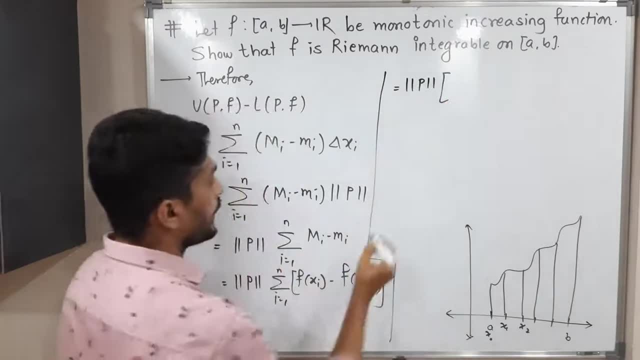 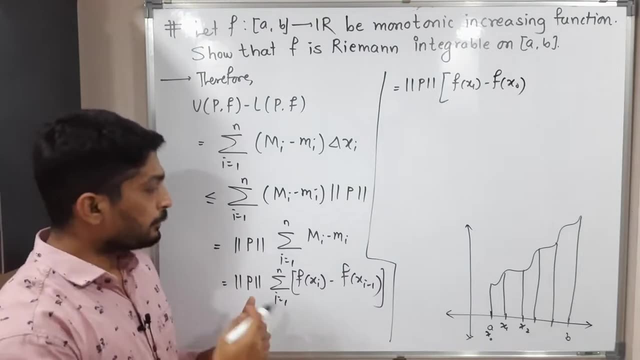 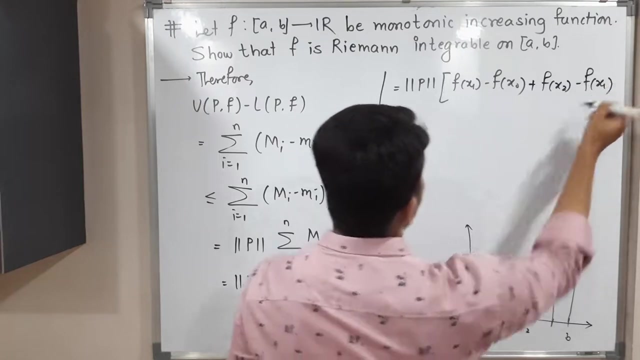 to norm p. Okay, So let us put i is equal to 1.. So f of x1 minus f of x0, since 1 minus 1, 0.. I'm going to put i is equal to 2.. So it will be f of x2 right minus f of x1, 2 minus 1, 1.. I'm going to 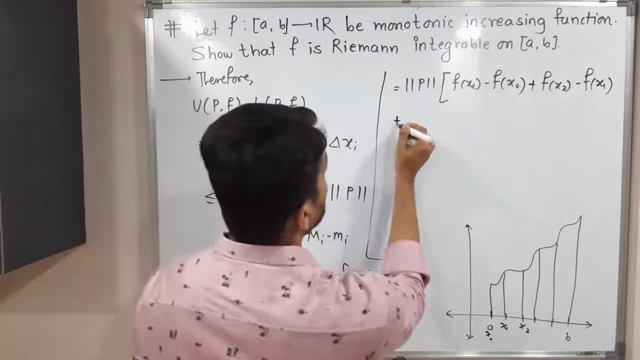 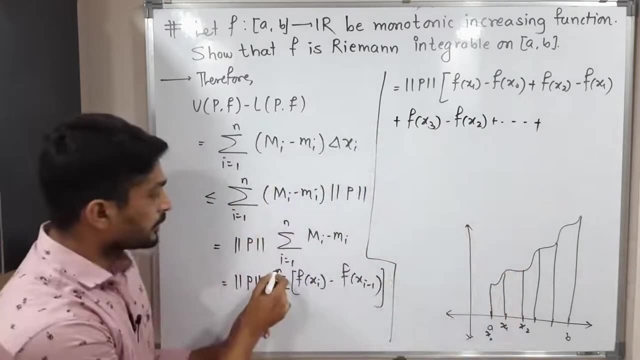 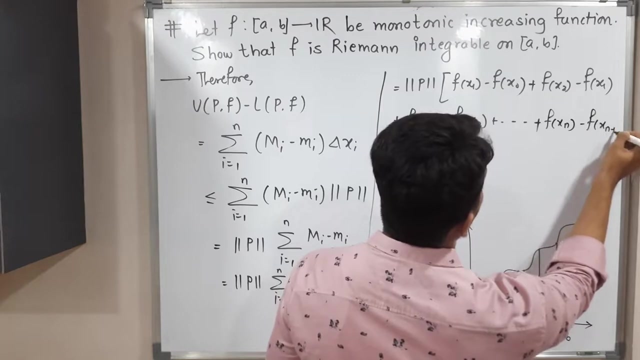 i is equal to 3 now. So plus f of x3.. Minus f of x2, and so on. At the end we have to put: i is equal to n. Then we will have f of xn minus f of xn minus 1.. Tell me, can we cancel anything here? Yes, definitely This f of x1. 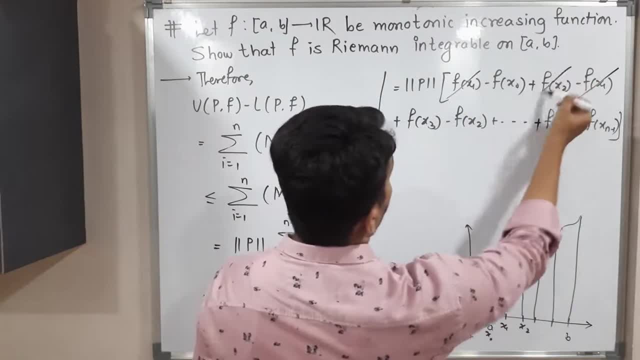 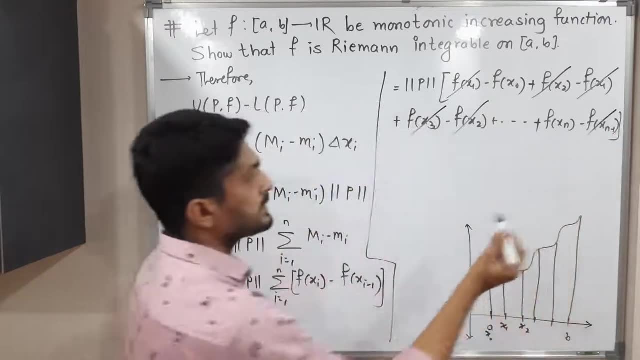 and minus f of x1 will get cancelled. f of x2 and minus f of x2 will get cancelled. Similarly, that f of x3 will get cancelled with minus f of x3 and minus f of x2 will get cancelled with minus xn. minus 1 also will get cancelled with. One term will be here having positive sign, So we'll 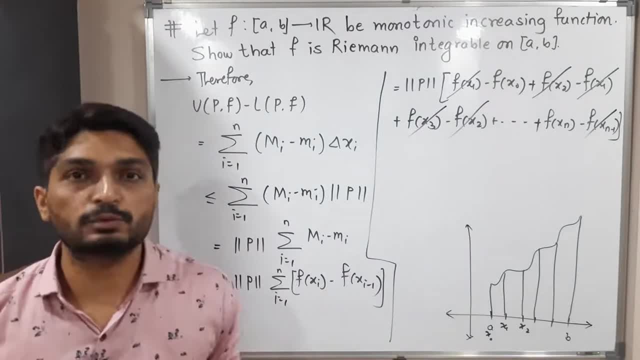 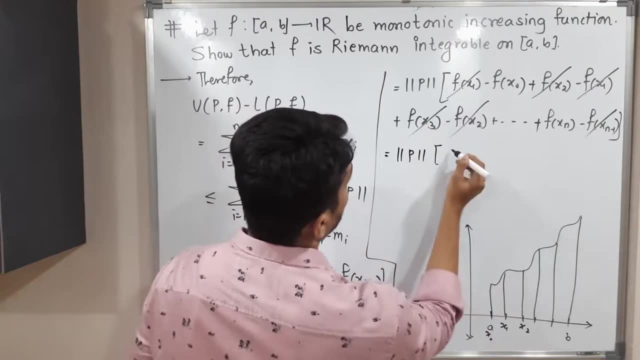 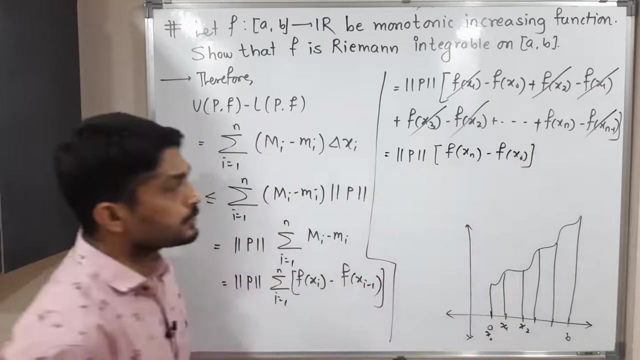 get cancelled. What I want to say, just first and last terms, will be there, Remaining. all terms will get cancelled. So therefore we will have norm p. Okay, What is the first term? Sorry, last term, f of xn and the first term having minus sign, f of x0.. Right, So f of xn. xn means last. 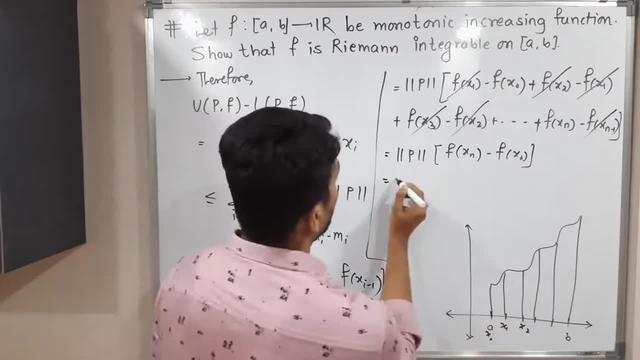 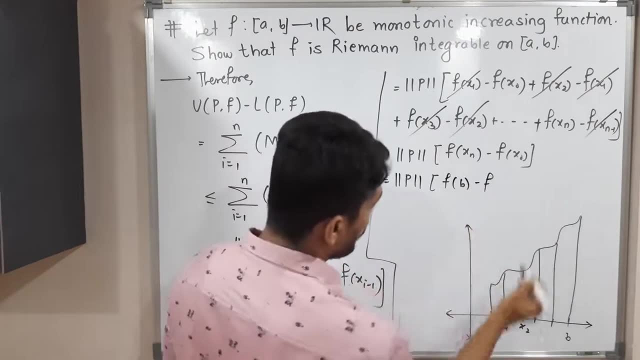 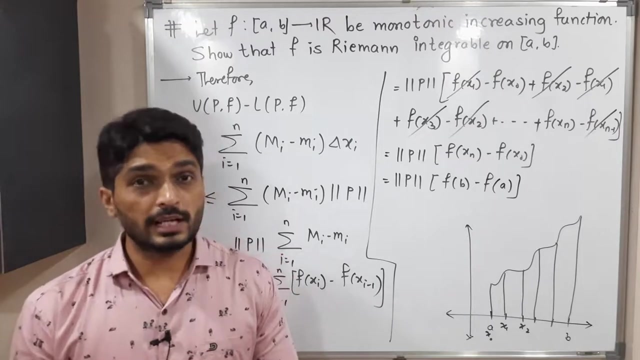 term. That means b Getting. So that is nothing. but let me write norm p: F of xn means f of b and f of x0.. x0 means a, So this is a. But do you remember that equation star? Equation star says norm p is less than epsilon by f of b minus f of a. 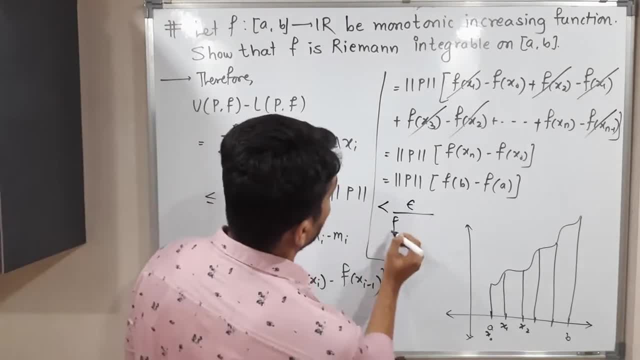 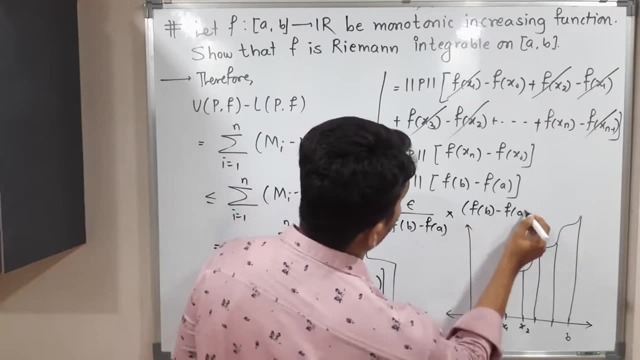 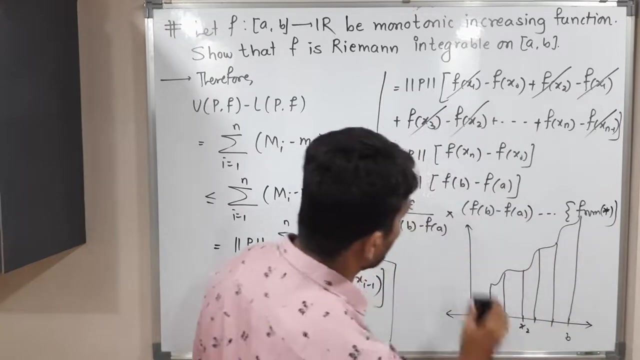 Let me use that. So this is less than epsilon by f of b minus f of a And this bracket also. we have f of b minus f of a. Let me mention from Star: Okay, Let me remove this diagram. It is not required now, Okay, So we will have some. 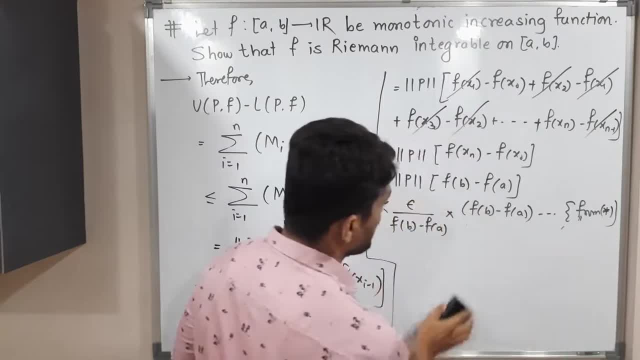 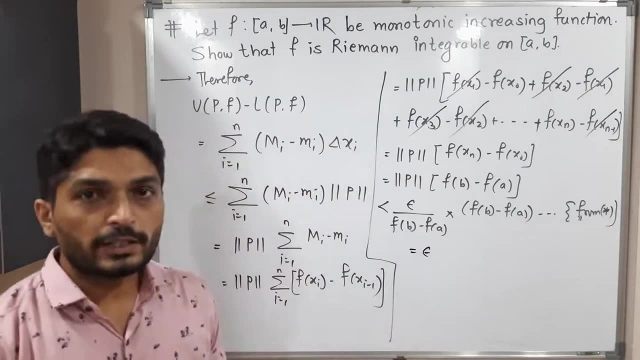 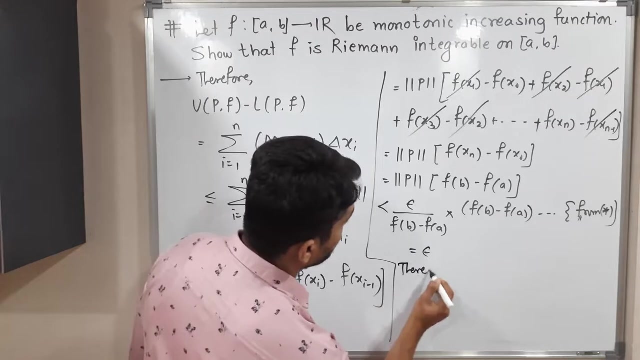 more space to solve this example? Yes, It is. See, these two brackets will get cancelled to each other, So we will have epsilon. Do you remember? we started with what We started with upper sum minus lower sum And what we got: less than epsilon. So let me mention, Therefore, Therefore, 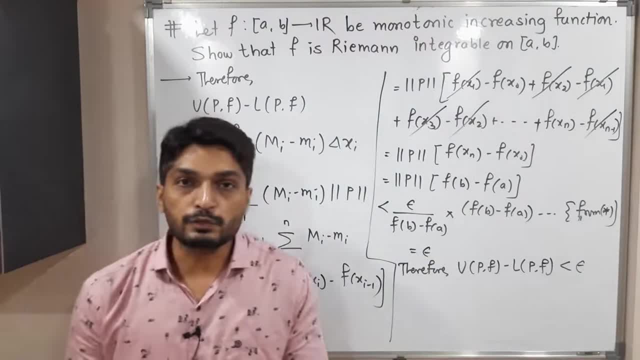 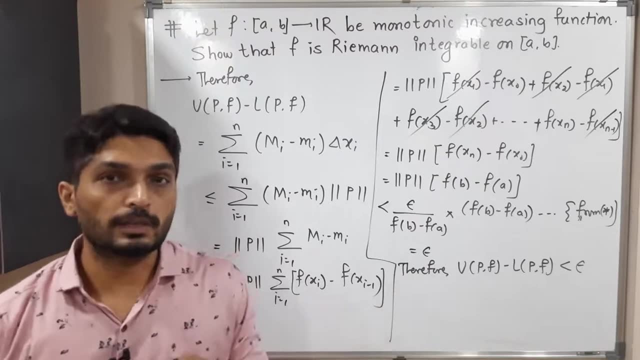 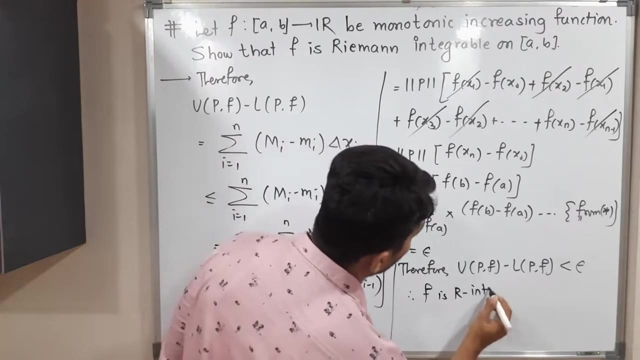 It is less than epsilon. So already in previous video we have studied Riemann criteria. Okay For integrability, And using that criteria we can say: yes, function is Riemann integrable on closed interval. a, b, So therefore f is R integrable, R integrable on closed interval. 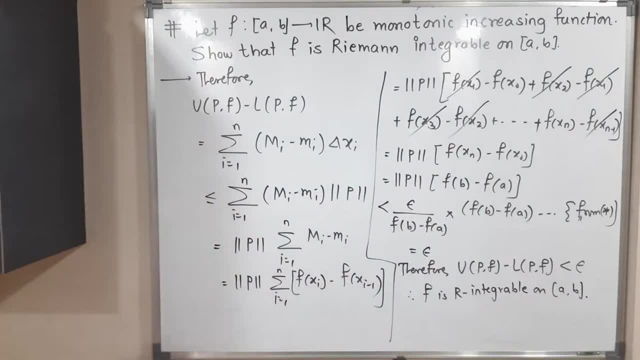 a, b. So therefore we can say that function. if it is monotonic, then it is Riemann integrable. So make a screenshot of it And stop. Thank you, Bye, bye.